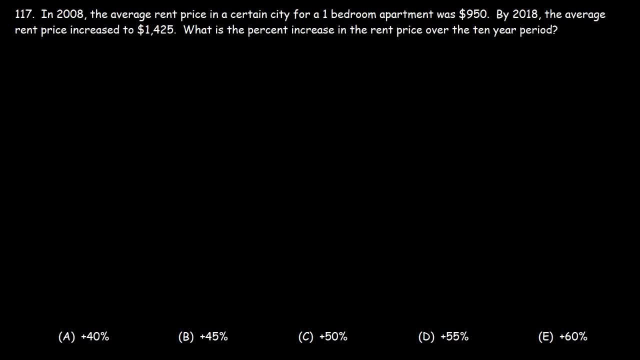 Number 117.. In 2008,, the average rent price in a certain city for a one-bedroom apartment was $950.. By 2018, the average rent price increased to $1,425.. What is the percent increase in the rent price over the 10-year period? There's a 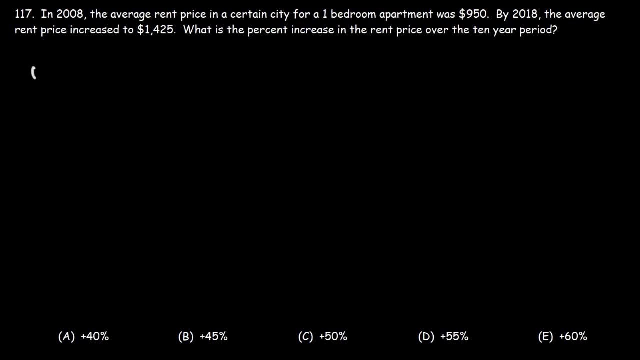 formula in which we can calculate the percent change. Here it is. The percent change is equal to the new price minus the original price, divided by the original price times 100%. So the new price is $1,425.. The original price is $950. 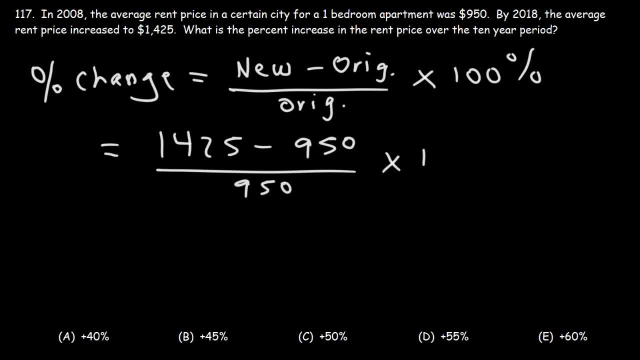 and we're going to divide it by $950 again. So $1,425 minus $950.. Let me re-type that again: That's going to be $475.. Now let's divide $475 by $950. So that's 0.5. and then let's multiply that by a 100%, So the rent. 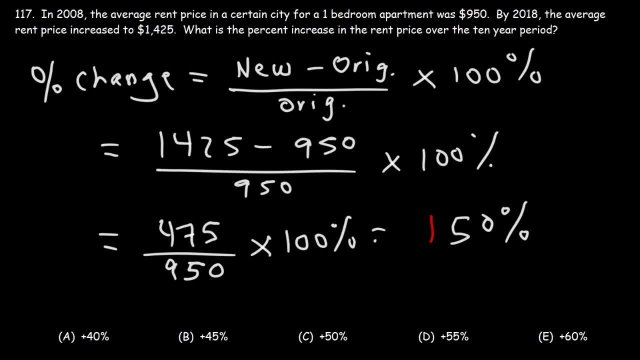 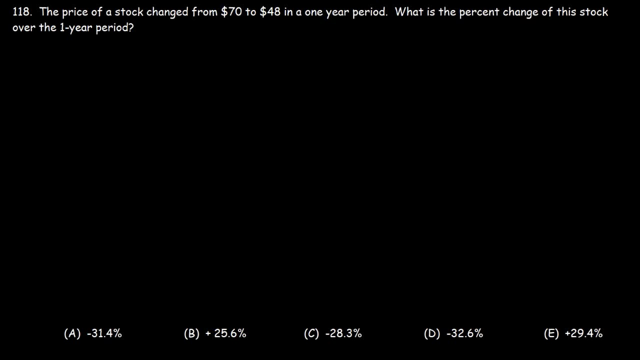 increased by $1,425.. increase by 50% over this 10-year period. Real estate tends to go up in value, but answer choice C is the correct answer 118,. the price of a stock changed from $70 to $48 in a one-year period. 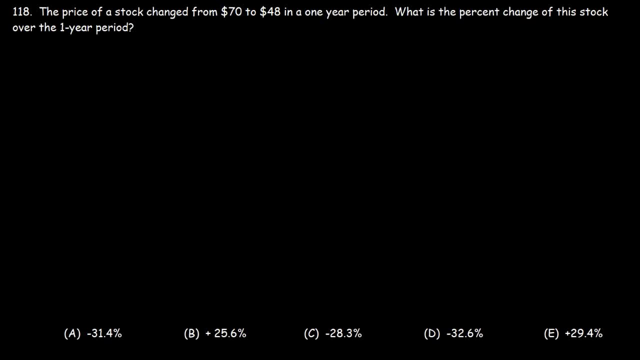 What is the percent change of this stock over the one-year period? So we're going to use the same formula. The percent change is going to be equal to the new value, which the new value is $48 minus the original value of $70, divided by the original value times 100%. 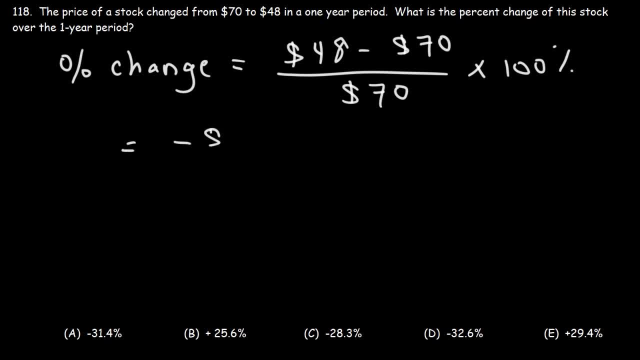 So 48 minus 70,, that's negative $22.. Okay, Okay, Okay, Okay. So now let's divide negative 22 by 70, and then let's multiply that by 100%, So you should get negative 31.4%, and of course this is a rounded answer. 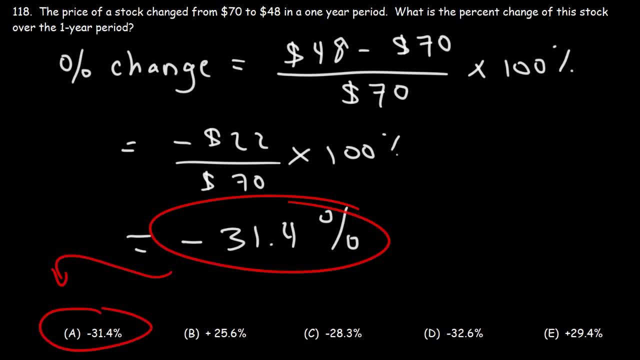 So answer choice A is correct. So the negative sign tells us that the stock decreased in value. If we had a positive sign, it would indicate a percent increase, where the stock would increase in value, But a negative sign would indicate a decrease in value. 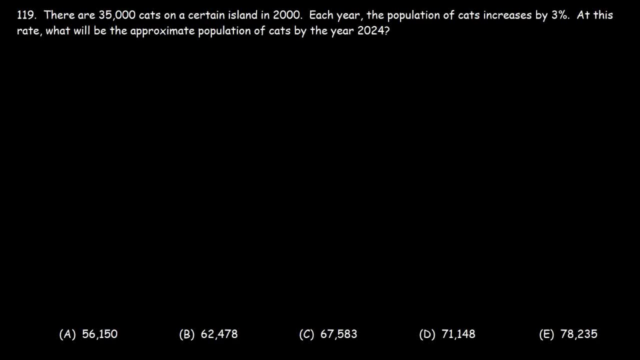 So the negative sign indicates a percent decrease. Number 119,: there are 35,000 cats on a certain island in 2000.. Each year the population of cats increases by 3%. At this rate, what will be the approximate population of cats by the year 2024?? 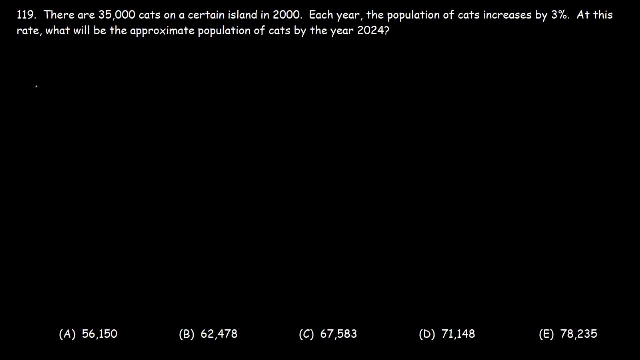 Well, let's find out. So let's write a formula. Let's say the population with respect to time is represented by the major- But I'm going to write an approximate time- of cats is represented by the function p of t. now this is going to equal the initial amount times, basically. 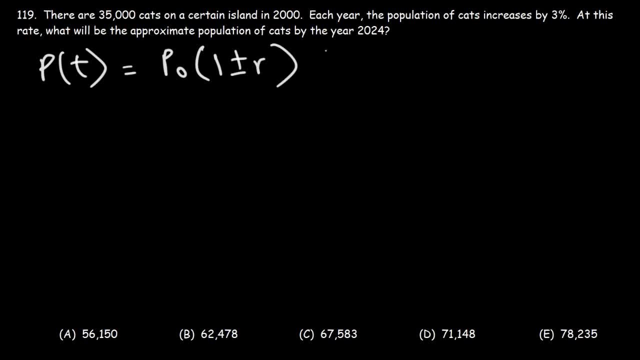 1 plus or minus r. raised to the t where t is in years, the initial amount of cats p 0 is 35 000.. r is three percent. now notice that it increases by three percent. so we're going to use the positive sign. thus this is going to be 1 plus r 3. if you divide that by 100 is equal to 0.03 as a decimal. 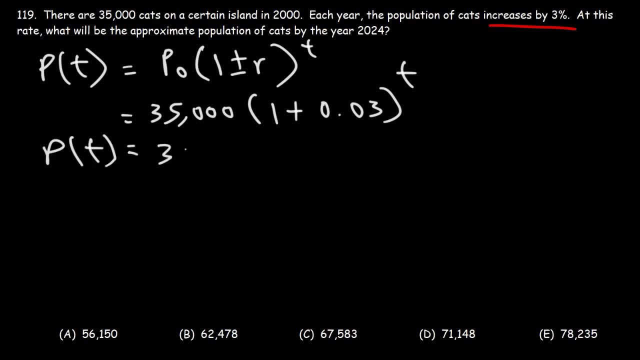 so thus we have the formula for the population of the cats. it's 35 000 times 1.03. raised to the t, now t is 0, corresponding to the year 2000.. so by the year 2024 t should be equal to 24.. 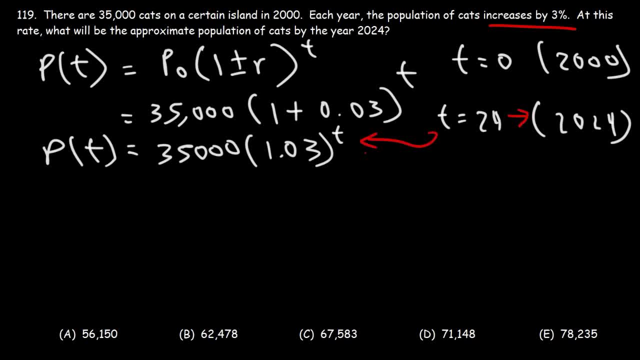 so let's go ahead and plug this in. so we're calculating p of 24, which is 35 000 times 1.03 raised to the 24th power, and so you should get seventy one thousand one hundred forty seven point seven nine, so rounding that to nearest whole number. 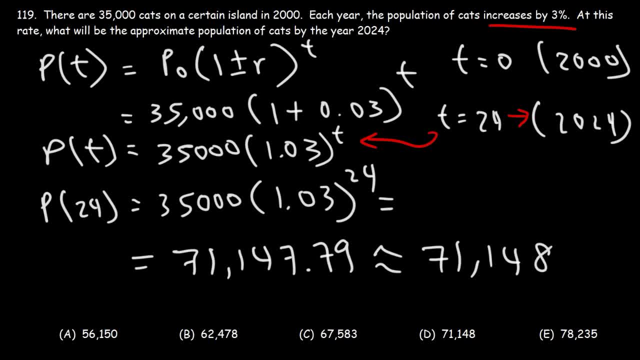 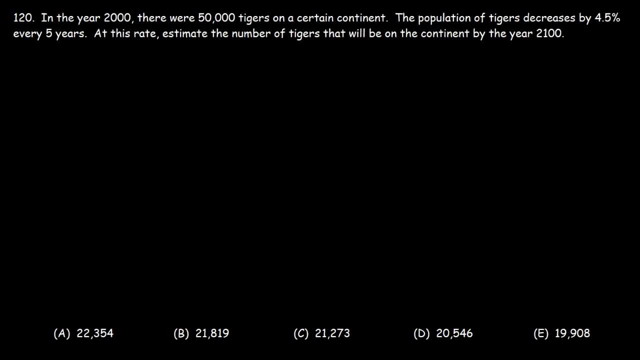 that's seventy one thousand one hundred forty eight approximately, which means answer. choice d is the answer number 120. in the year 2000 there were fifty thousand tigers on a certain continent. the population of tigers decreases by four point five percent every five years at this. 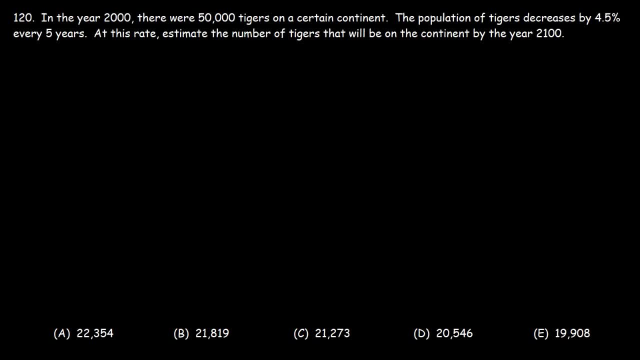 rate estimate the number of tigers that will be on the continent by the year 2100.. so let's start with this formula again. so p of t is equal to p initial times one plus or minus r raised to the t. now this formula is going to be different because t is basically the number of years. however, 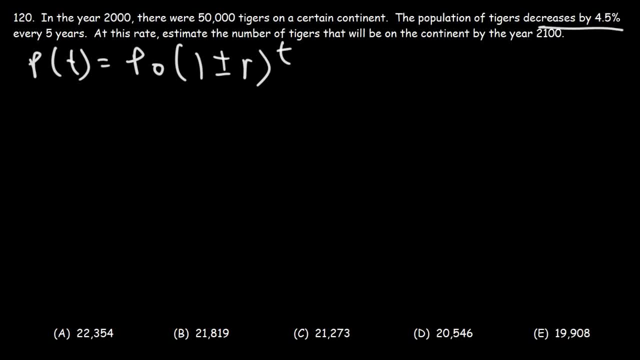 notice that the population decreases by 4.5 percent every five years. so in order for t to be the number of years, we need to divide it by n, where n is the number of times the population is compounded by a decrease of 4.5 percent. 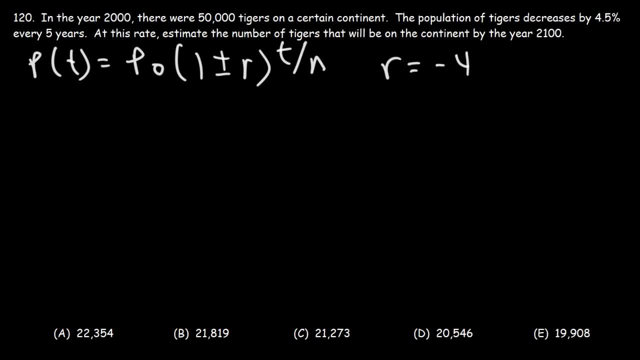 so in this example, r is going to be negative 4.5 percent, or you can think of r as being positive 4.5, but we're going to use the negative sign now. the second thing is n is 5. because it's going to change by r every five years. 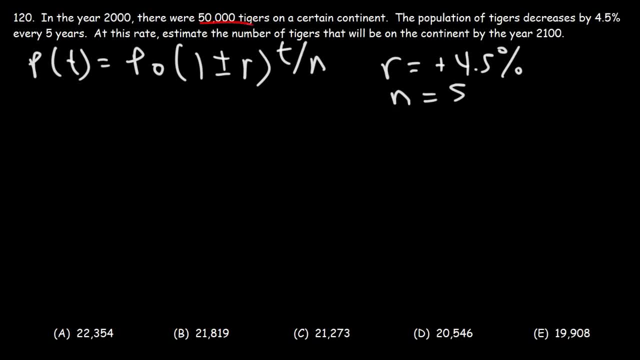 now the initial population, p 0, that's going to be 50 000.. so the formula is going to be: fifty thousand times one minus now 4.5 percent. if we divide that by 100 that's 0.045, and then we're going to raise it to the t. 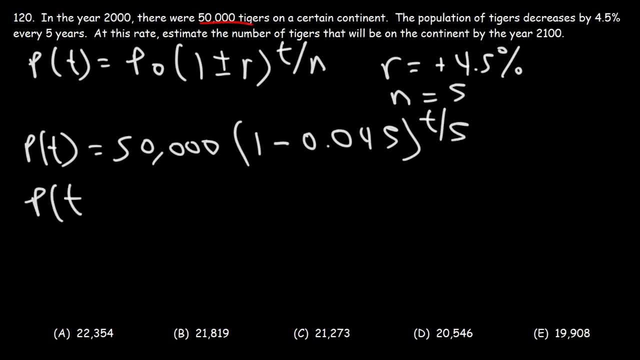 by 5.. So we have: P of T is equal to 50,000.. 1 minus 0.045, that's going to be 0.955 and that's raised to the T over 5.. Now what is T in this example? In the year 2000, T is: 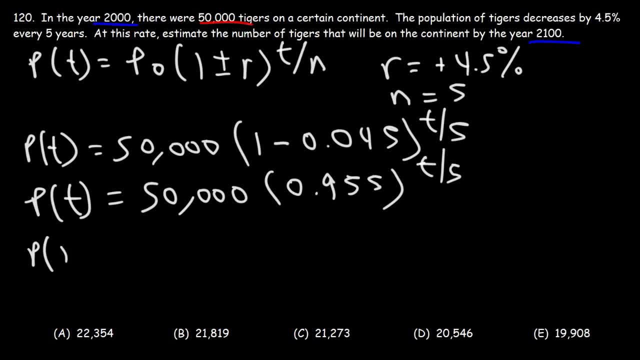 0. But by the year 2100, T is going to be 100. So the population decreases by 4.5% every 5 years. So in a 100 year period it's going to decrease by this amount 20 times As you. 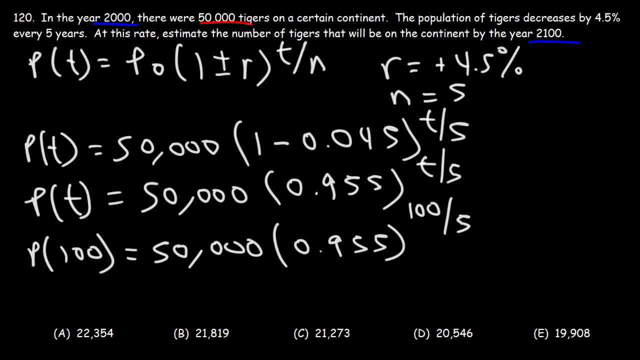 can see: 100 divided by 5 is 20.. So this is going to be 50,000 times 0.955.. Raised to the 20th power, And so the population by 2100 is going to be 19,908 tigers rounded. 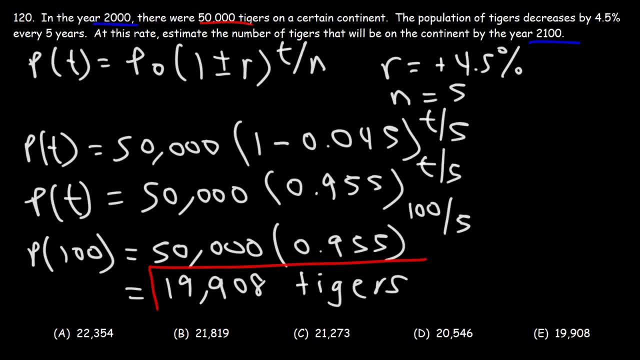 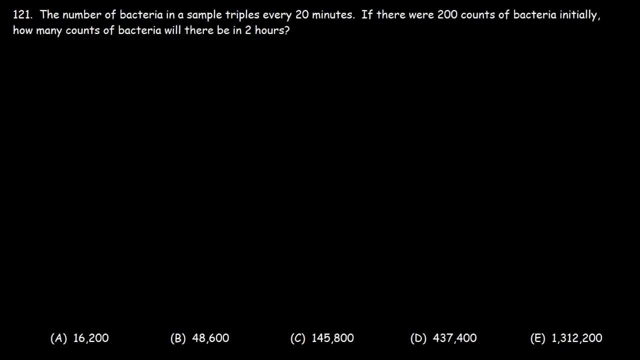 to the nearest whole number. So that's how we can answer this particular type of question. Answer choice E is the answer Number 121,. the number of bacteria in a sample triples every 20 minutes. So how many counts of bacteria initially, How many counts of bacteria will there be? 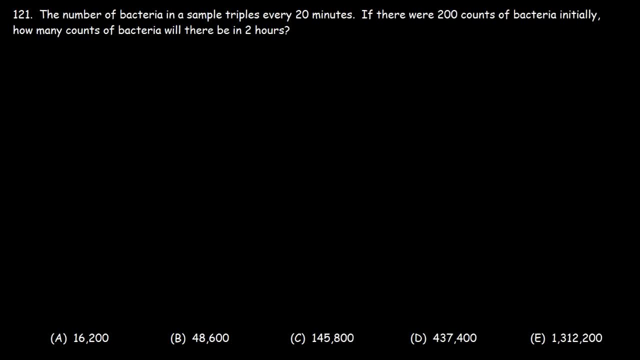 in two hours. Well, let's find out. So the population of bacteria is going to equal the initial amount. In this case, I'm going to say let's use the letter X raised to the T over N. The initial amount is 200.. X would be the number of times let's say if it double. 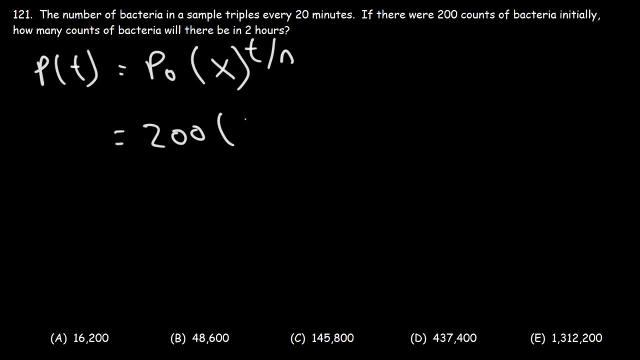 or triples or quadruples. Because it triples, X is 3.. T is going to be the time in minutes. Notice that it triples every 20 minutes. So N is going to be 20 or 20 minutes. So because N is in minutes, T has to be in minutes. 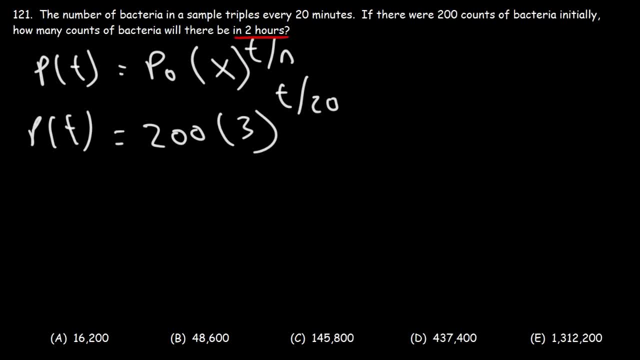 Now we want to find out how much bacteria there's going to be in two hours, So we need to convert that to minutes. There are 60 minutes in one hour, So this is going to be 2 times 60. So that's 120 minutes. 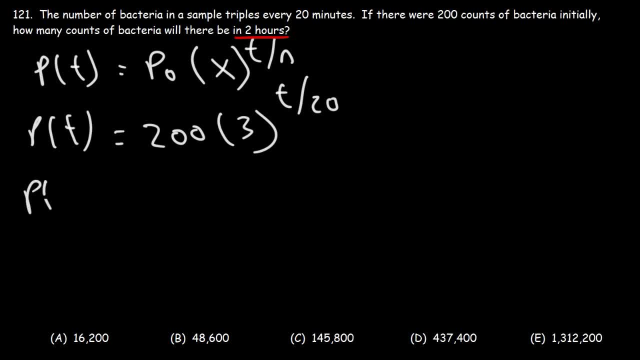 So that's T. So let's calculate the population of bacteria 120 minutes later. So it's going to be 200 times 3 raised to the 120, divided by 20.. 120 divided by 20 is 6.. So in a two hour period the number of bacteria is going to triple six times. because it triples. 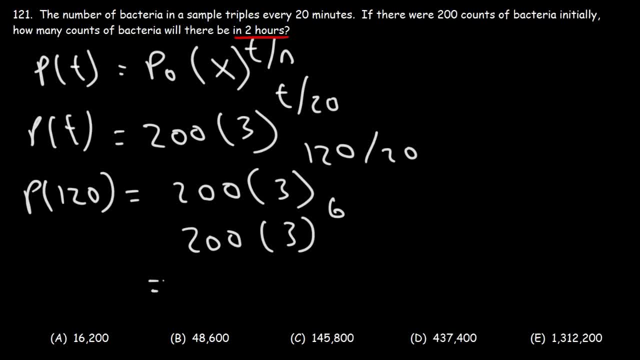 every 20 minutes. So 200 times 3, raised to the 6th power, This is going to be 145,800.. So that is the population of the bacteria that's going to be present two hours later. So answer choice C is the. right answer.